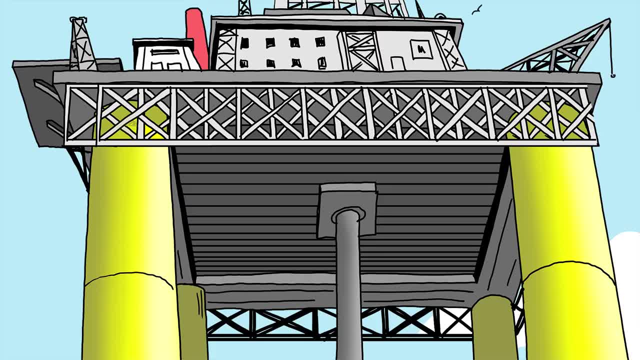 Got it. The Gulf of Mexico has one of the biggest oil reserves on the planet. That's why there are so many companies out here drilling. How do they know where to drill? That's what those ships are doing: They're drilling. They're drilling. 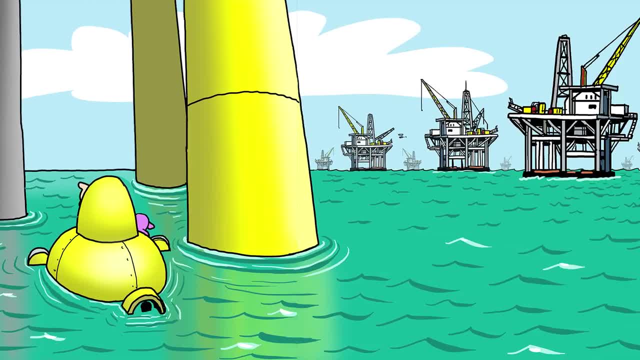 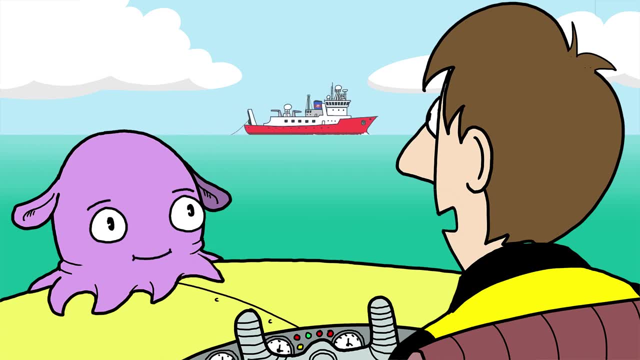 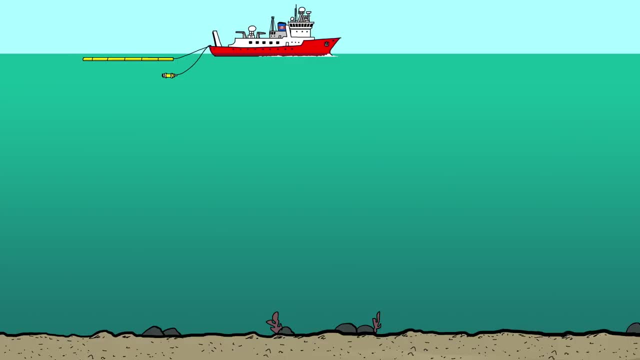 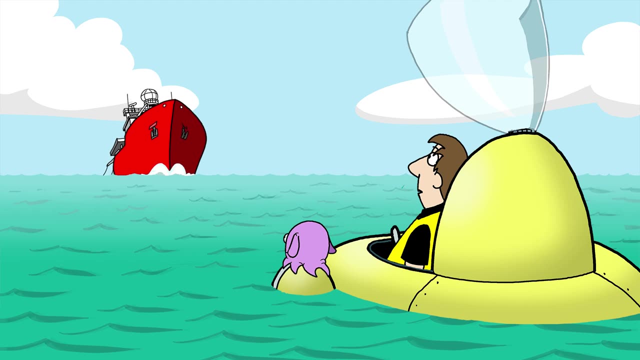 It's used to find the oil and gas reserves. How's it do that? It shoots loud blasts which hit the bottom and reflect back to the ship. With the right equipment, they can locate buried oil and gas deposits. Look, They're making another pass. 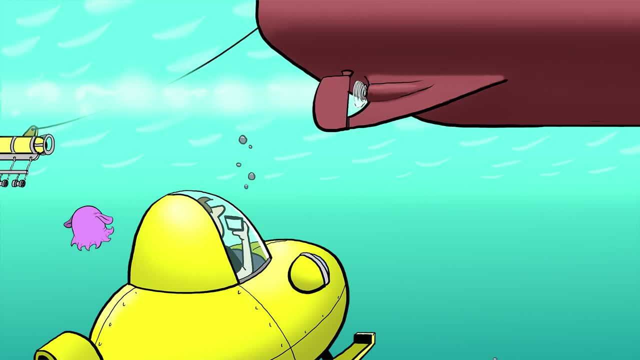 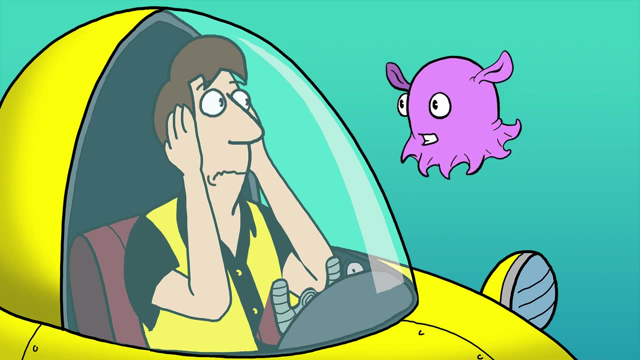 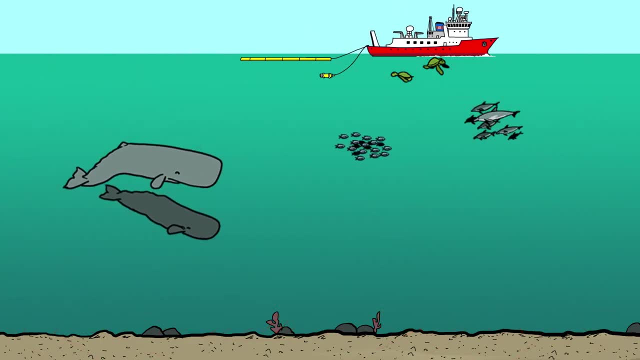 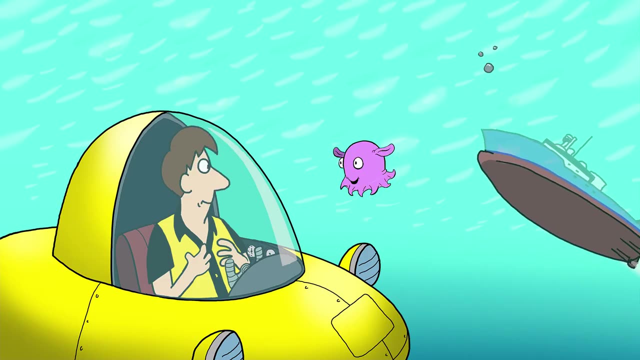 Whales and dolphins live in a world of sound. These blasts totally disrupt their ability to navigate, communicate and find food. Here comes that deep-sea trawler again. Let's head down to the bottom and see what's happening. Oh. 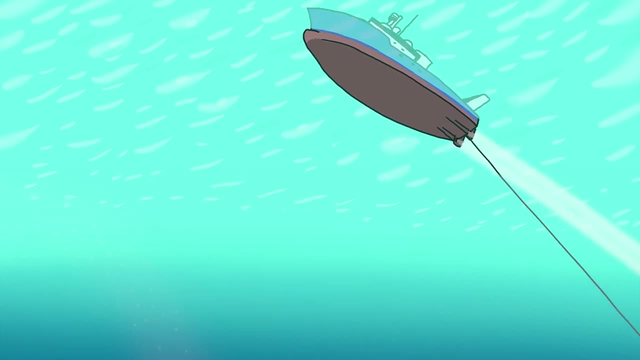 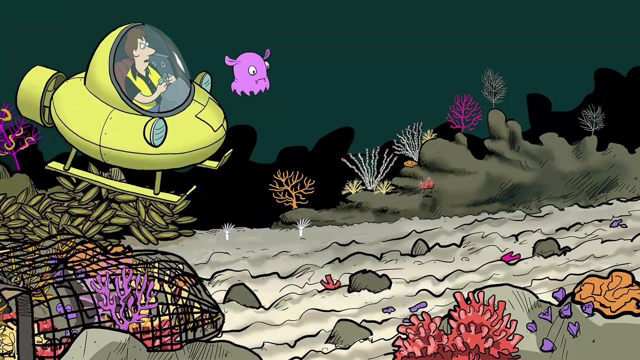 Okay, Good idea. They're catching fish and other creatures that live here. In a matter of seconds, they clear every living thing from the sea floor. That doesn't seem like a very smart way to catch fish By destroying their homes. No, it's not. 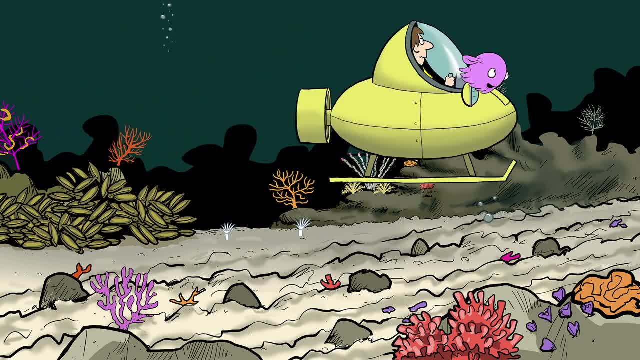 These ecosystems take hundreds of years to recover, And that's if they recover. Remember that big oil rig we saw up on the surface? This is what the other end looks like. So now you're going to tell me this is bad too. It's not as easy as all that. Oil and gas production are a big part of the economy around here And people need energy to- Power our cell phones and cars and, well, just about everything we do. right, You got it. 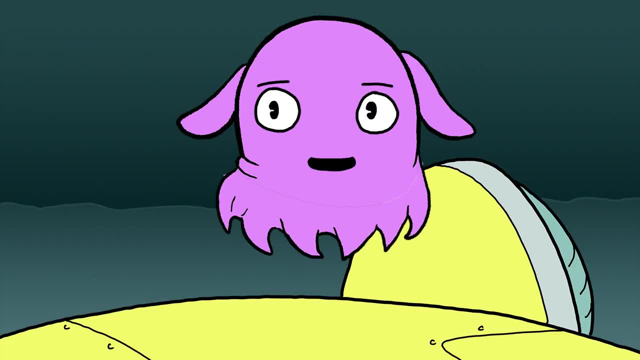 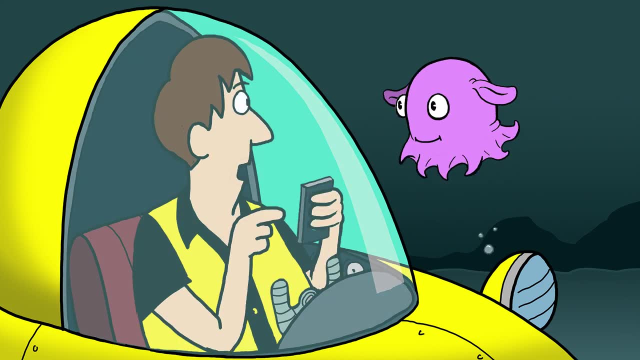 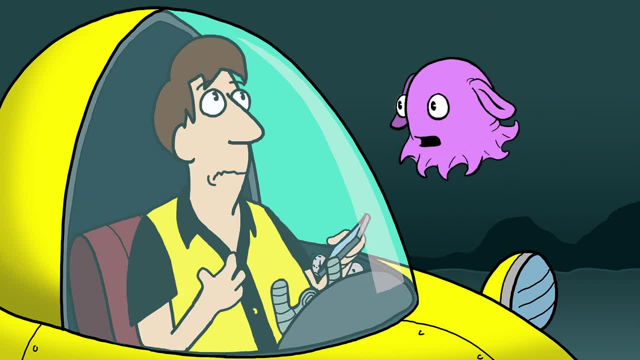 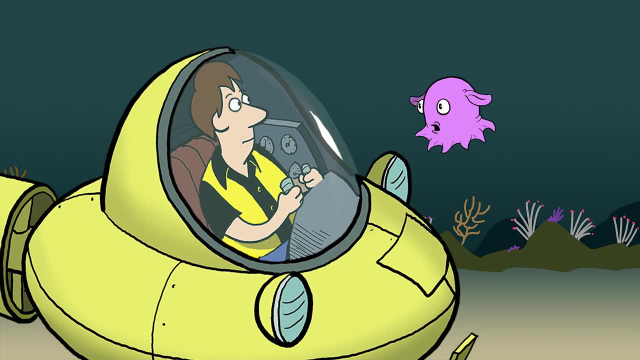 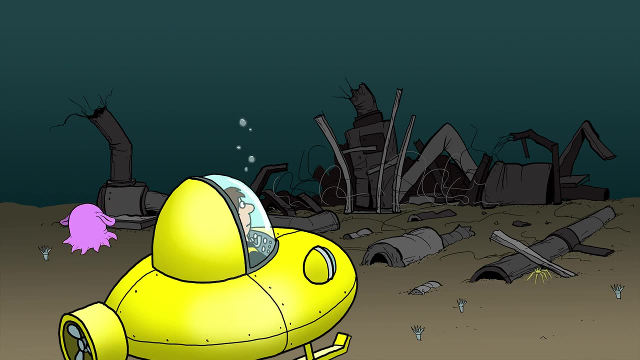 That's right, And chemicals that are used in the drilling process can pollute the water, And every now and then, accidents happen. This is what's left of the deep water horizon rig, which caused one of the biggest oil spills in history. I remember when this happened. 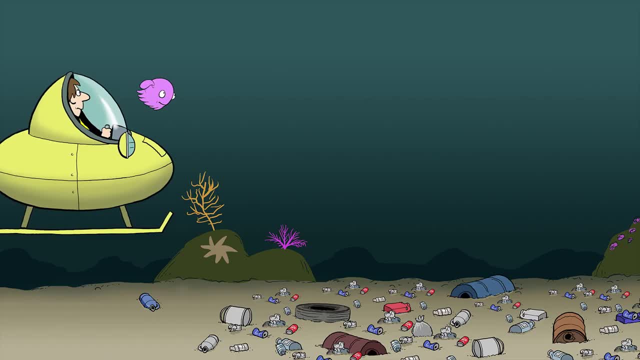 It was a disaster For the ocean And for people too. Is that trash? How did it get way down here? We're like a mile deep in the ocean. You can find trash anywhere. We're like a mile deep in the ocean.